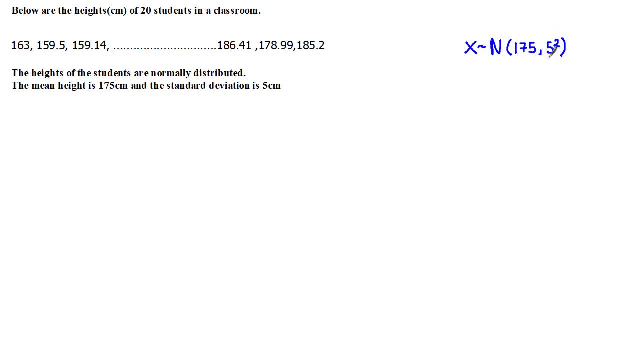 But what we write here is 5 squared, which represents the variance. In statistics we use a capital X to represent a random variable and use a lowercase x to represent the different values that the random variable can take on. So here I've just labelled some of the heights, in no particular order, with lowercase x sub 1 up to x sub 20.. 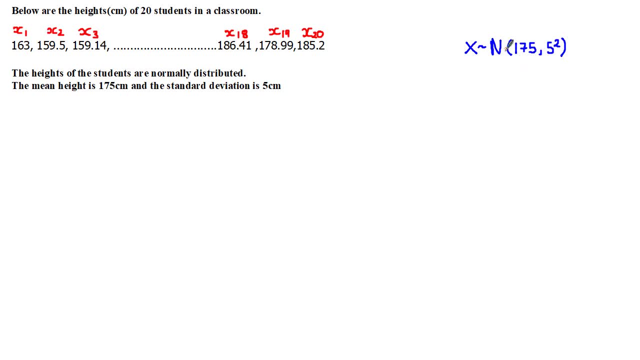 The mean given to us in this question was 175 centimetres, And there's a special name for this mean, And it's x sub 1.. And it's called the population mean, which is a true mean of the data, Since this distribution is normal. we can also illustrate this distribution using a bell shaped curve, where the population mean would be at the centre. 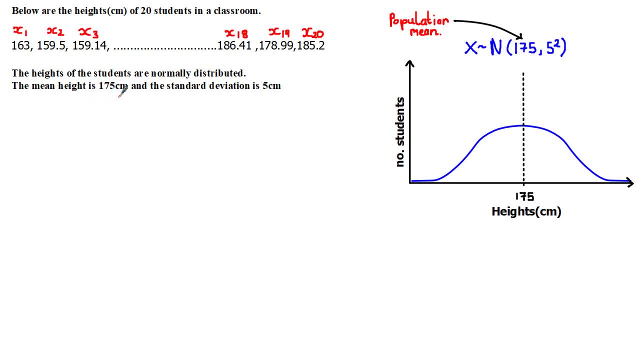 Now, assuming we didn't know what this mean was, but we wanted to estimate it by taking samples of the data, Well, the test statistic would be the sample mean, because it's the statistic that we'll be testing to give us the data. 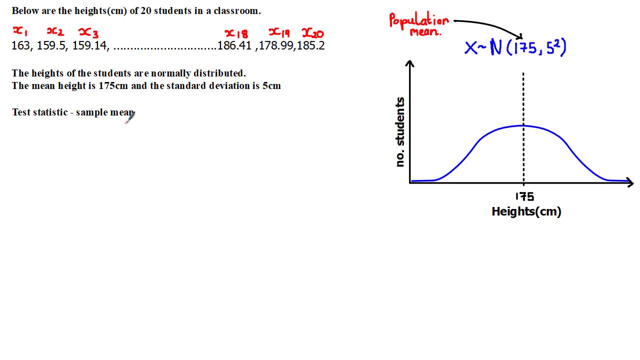 Now, in order to conduct the sampling method, of course we would need to choose a sampling size- n. OK, so assuming we chose n to be equal to 3 and we started taking random samples of this data, Well, if by chance we chose the first three values of the data, the mean, which I'll call x bar sub 1, would be equal to the sum of those values divided by 3.. 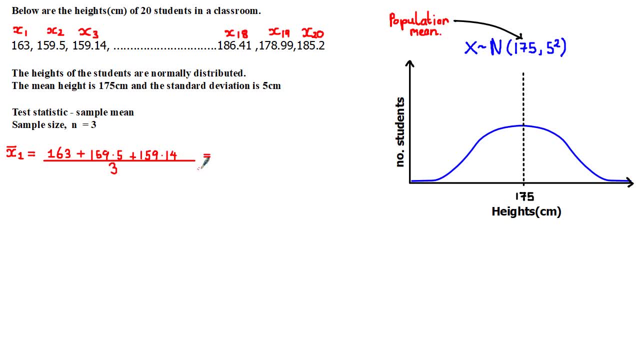 So, adding these values and dividing by 3, we get that the mean of this sample is 160.5 centimetres to one decimal place. And if, by chance, we happen to choose the last three values, well, the mean, which we'll call x bar sub 2, would be equal to the sum of those values divided by 3, which is equal to 183.5 centimetres to one decimal place. 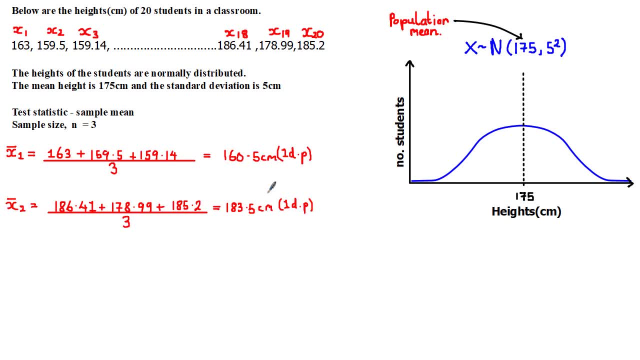 And do check these values in your calculator. Now what we've just calculated is that we've got x bar sub 2.. Now what we've just calculated are called sample means and they're used to estimate the population mean. We usually give them the notation x bar, but hopefully you can notice by just looking at these values that they're not very good estimates of the population mean, which is 175 centimetres. 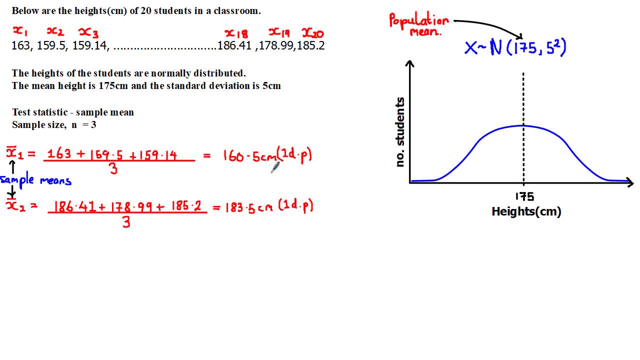 And mathematically we can also see that these values would lie outside one standard deviation away from the mean. since the standard deviation is 5 centimetres, One standard deviation away from the mean would be 175 plus or minus five. So you can clearly see that these values would lie outside of the range 170 to 180 centimetres and therefore shouldn't be taken as a reliable estimate for the mean of this data. 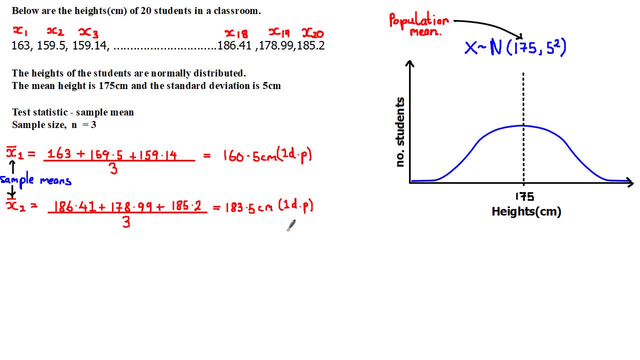 But what we do to make the sampling method more reliable is that we take more and more random samples of the mean, And if you were to take several, several more samples, you would get something called a sampling distribution of the sample means. now this might sound a little confusing, but all it is is a collection of sample means. 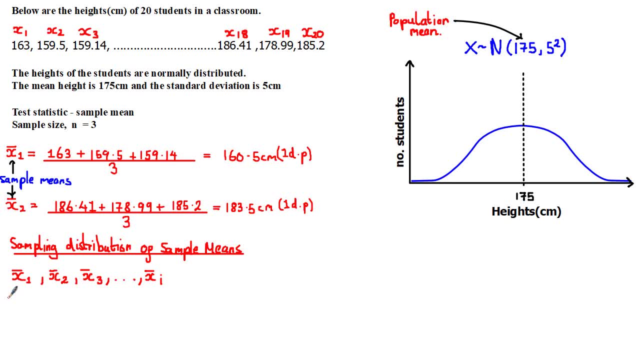 which form its own distribution, that we can write as a set of values, as you can see here: x bar sub 1, x bar sub 2, all the way up to x bar sub i, where i would be the number of samples we take from the original data. i've intentionally indexed up to i to show that 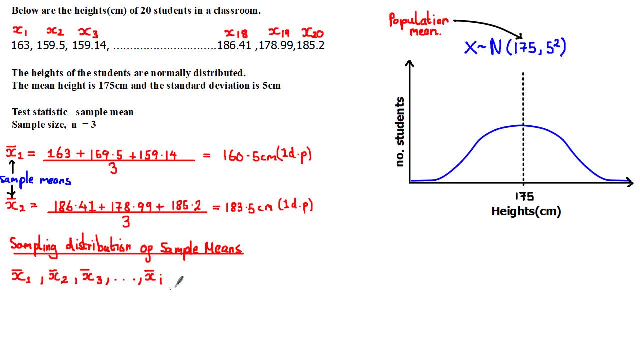 the number of samples is equal to i and not equal to n, which was 3, the sample size. okay, so that's a common misconception. so do take note of the fact that the number of samples is not the same as the sample size, n. we can use capital x bar to represent the distribution of. 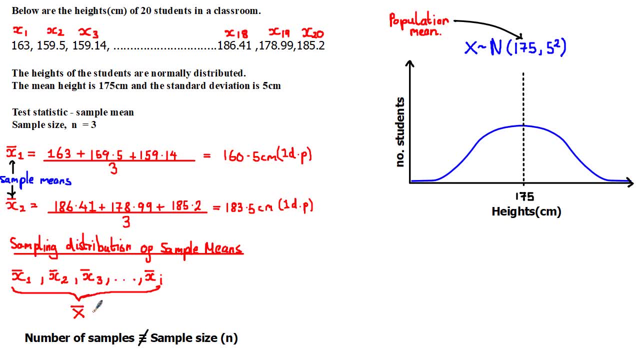 sample means. now this distribution is quite special. on the same graph. if we were to plot the distribution of sample means where the sample size n was equal to 3, we would get a curve that looks like this, and what you would find is that the sampling distribution of the sample means is also normally. 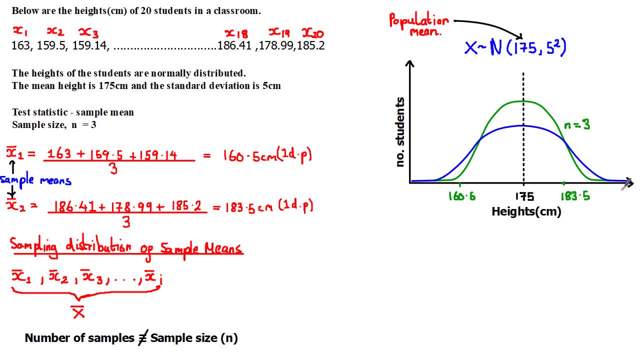 distributed, which means that you can calculate its mean and standard deviation, and what you'd notice is that the mean is equal to the sample size n and the sample size n is equal to the mean of the sampling. distribution will always be equal to the mean of the original distribution. 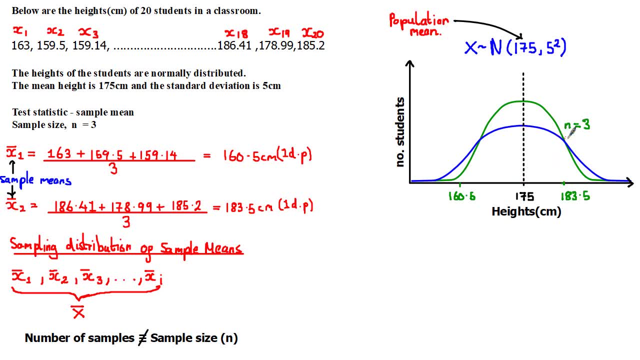 which was the blue curve. but provided the sample size is greater than one, the standard deviation of the sampling distribution of sample means will always be smaller than the original distribution. and this is really what we expect, because when we take more samples of our data, we expect to get a better estimate of the population. 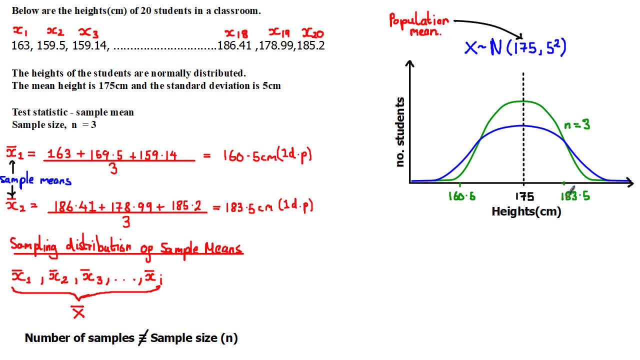 mean and in the context, a better estimate means a smaller spread of the data around the mean, otherwise known as the standard deviation. If we were to increase the sample size to say n equal to 16, in other words, for each sample in the data set we took the mean of 16 values. 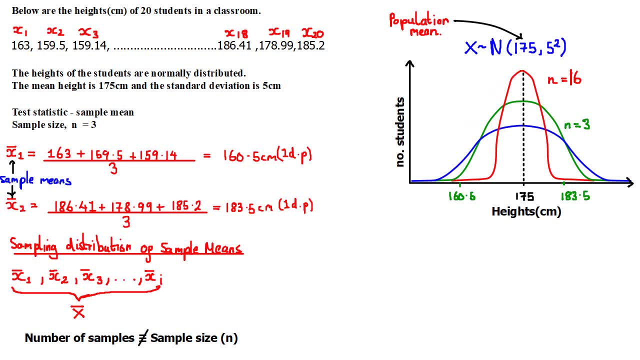 the sampling distribution of the sample means would have the same mean but an even smaller standard deviation. and this leads us to an important result. If a random variable, x, which represents the population, is normally distributed with a mean mu and a variance of sigma squared, then x bar the variable that represents the sampling distribution of sample means. 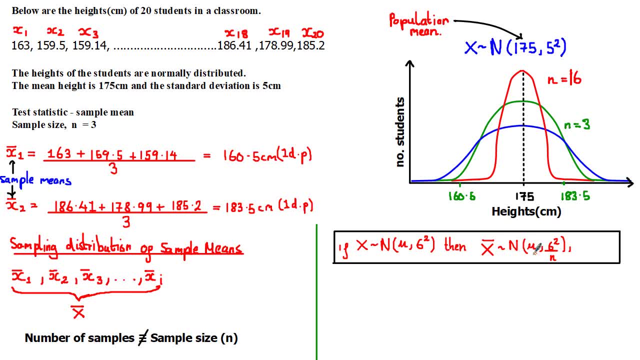 will also be normally distributed with the same mean as the population mean, but the variance would be equal to sigma squared over n, less than the population variance, and therefore the standard deviation would be sigma divided by the square root of n, which is just the square root of the. 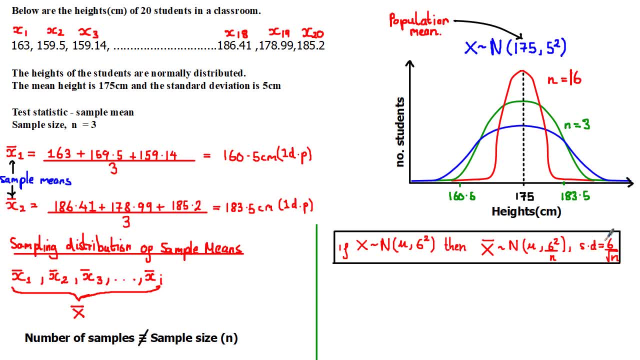 variance and from this result we can see why the standard deviation of the distribution of sample means becomes smaller when n, the sample size gets larger, which would make this fraction smaller. So from this example, if we let x represent the heights of students in the class, or, then we can say that the mean of the sample means, which we can call mu sub x bar, is equal to. 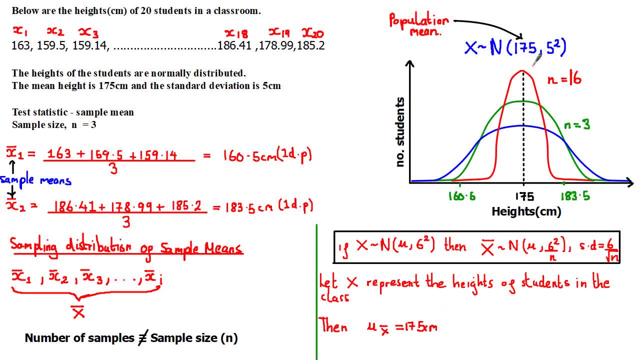 175 centimeters, the same as the population mean, and the standard deviation of the sample mean, which we can call sigma sub x bar, is equal to 5 over root 3, where n, in this case, would be equal to the sample size, which was 3.. and this is equal to 2.9 centimeters to one decimal place.